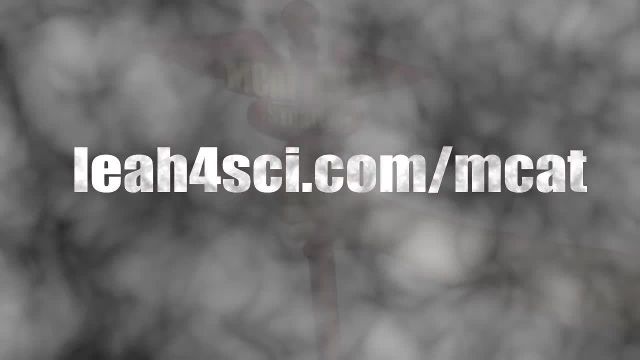 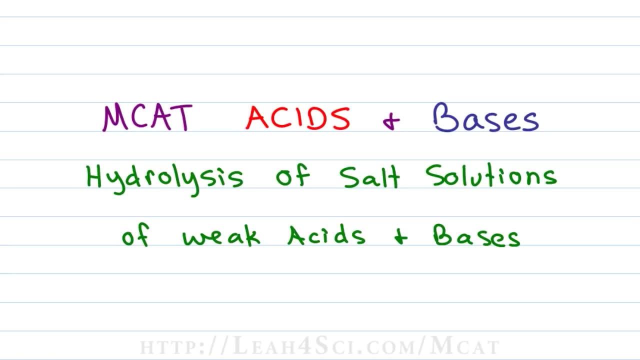 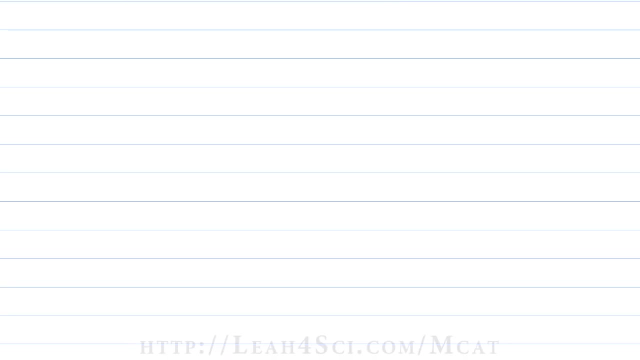 Leah here from leah4scicom, slash mcat, and in this video we'll look at the hydrolysis of salt solutions, particularly the solutions of weak acids and weak bases. To understand how a dissolved salt will impact the pH, you must remember what happens when an acid or 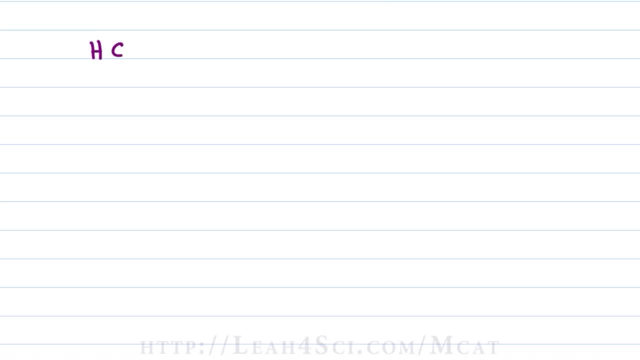 a base dissociates in solution. If we have a strong acid like HCl, it'll dissociate nearly 100%. to give you H plus and Cl minus ions in solution. A strong acid wants to dissociate. that means it'll form a weak conjugate base that does not want to grab that H plus and 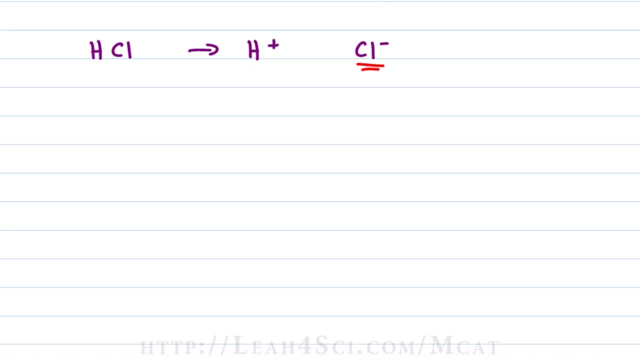 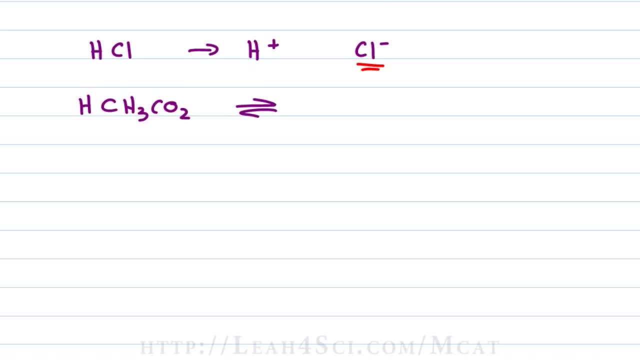 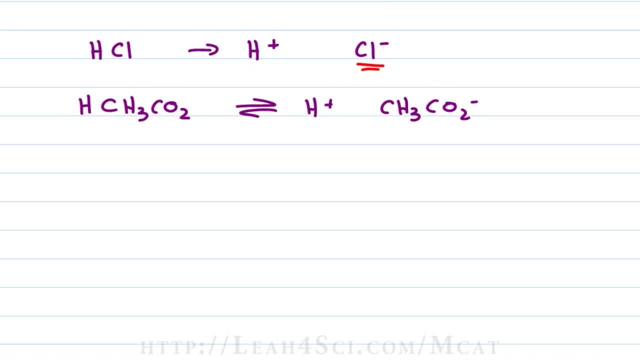 remain in solution as a spectator. Some of the acetate will grab that H plus and reform acetic acid. That's why we have the 2 way arrows to show that it's in equilibrium. So now what happens if you dissolved a salt of the conjugate in solution? If I take a salt, 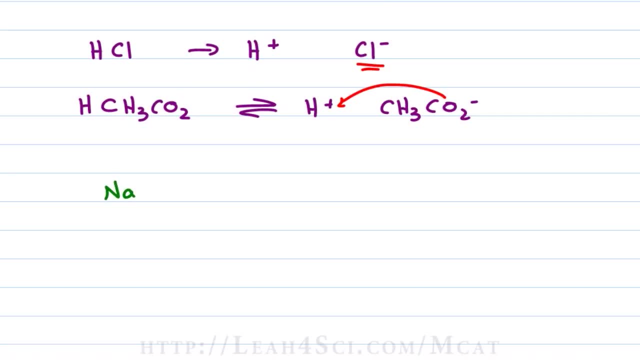 with a cation that is unreactive, like Na plus, and I dissolve NaCl in solution. This will break up to give me Na plus and Cl minus. These ions are spectators, they're not reactive, they won't do anything to the pH. But if I take the conjugate of a weak acid like acetate and dissolve that as a 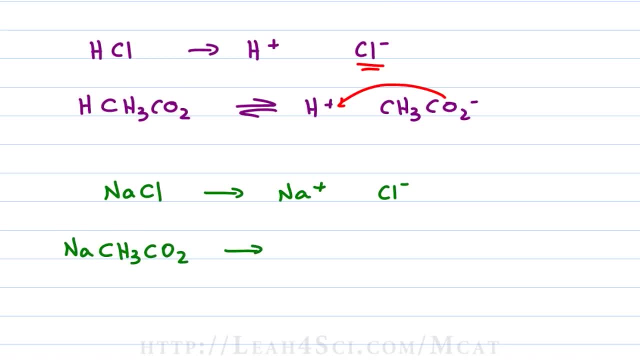 salt, for example sodium acetate. this dissolves to give me Na plus and acetate CH3CO2 minus. But just like the acetate from the acetic acid dissolving is not happy to stay 100% dissolved in the solution, the acetate from sodium acetate is also going to react. But if it can't react with, 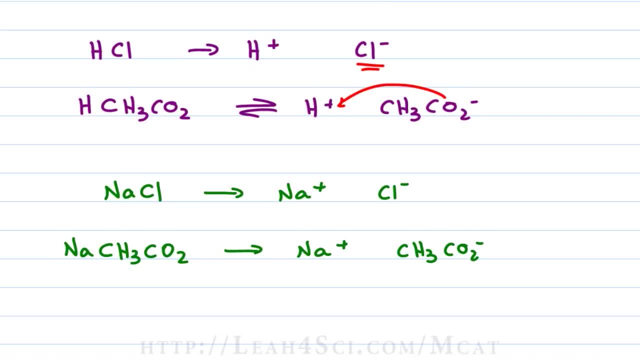 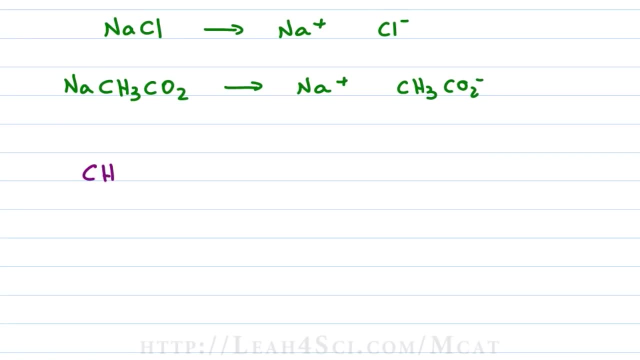 H plus that came off of acetic acid. it's going to react with water, pulling an H plus off that water molecule. If we write out the reaction, we'll see that we have CH3CO2 minus the starting base in solution reacting with H2O. 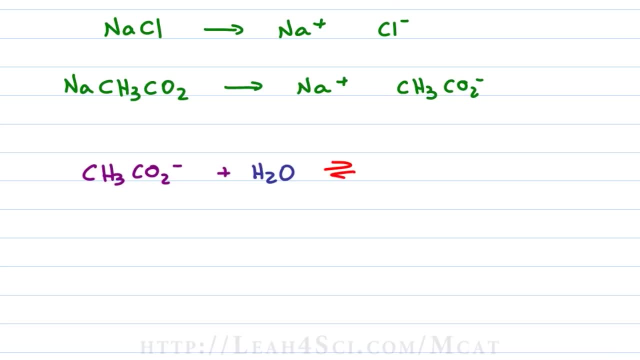 To give me an equilibrium that has acetic acid formed from the hydrogen of water and acetate, the starting base, and then OH minus. If we now analyze what we have in solution, we have some acetic acid, which will be an equilibrium between acetic acid and acetate, but we also have hydroxide. 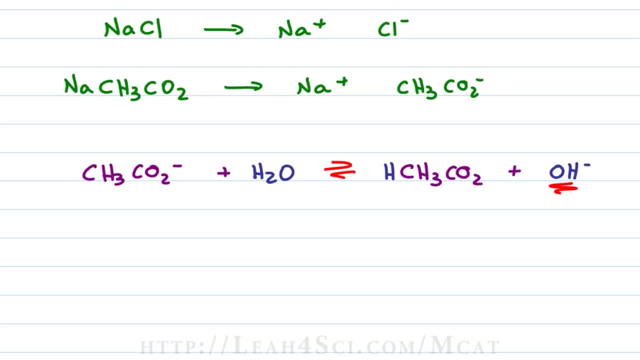 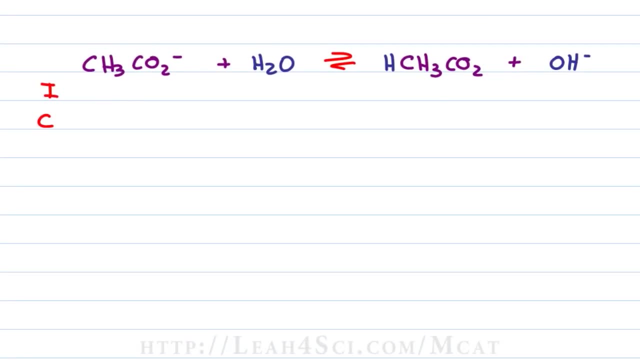 and hydroxide is a base, which means the pH of the solution will be greater than 7.. In fact, if you want to calculate this, you would have to write out a Ka expression and potentially write out the pH of the solution. But if you want to calculate this, you would have to. 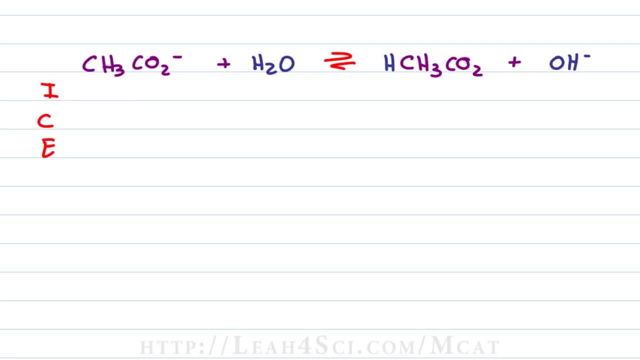 write out a Ka expression and potentially write out the pH of the solution and potentially write out the pH of the solution and potentially write out the pH of the solution and potentially set up a whole ice chart. We'd use the initial molarity of the sodium acetate as the starting concentration. 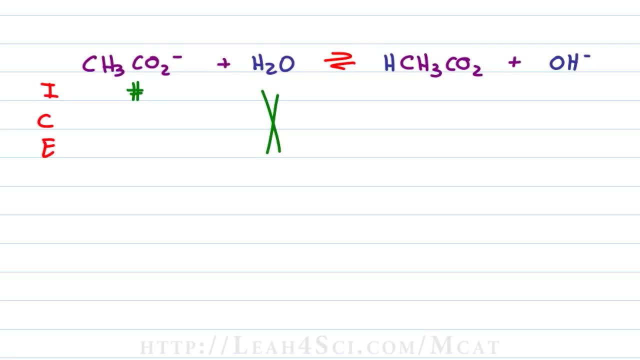 Water is a liquid, so we don't include it in a Keq expression and we'll assume 0 and 0 for acetic acid and hydroxide Acetate reacting with water will be X, so we'll show minus X for the acetate. 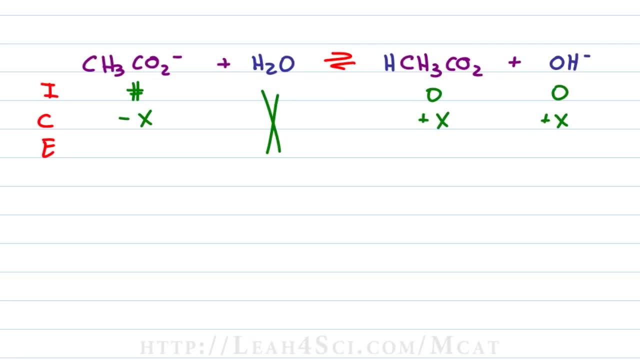 disappearing, plus X for the acetic acid and hydroxide for an equilibrium concentration of the molarity that we started with, minus X and then X and 0.. We're not going to go nuts solving this because remember the shortcut I showed you. in this case it's a base, so we'll write it as Kb for equilibrium expression is equal to X squared. 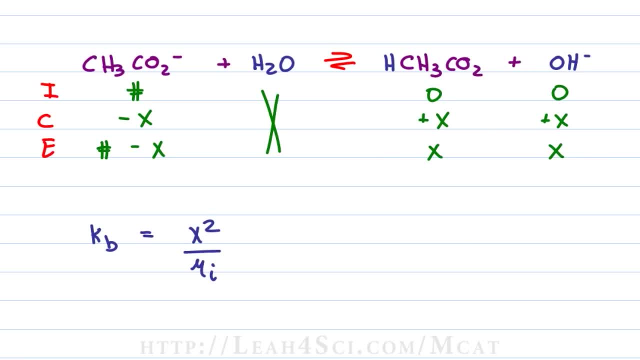 representing acetic acid and hydroxide divided by molarity: initial, because we're estimating that this is negligible and therefore drops out. But you'll notice that when we solve for X and X is equal to the OH- concentration, we have a basic solution. We'll get a pOH. we can turn that into a pH, but 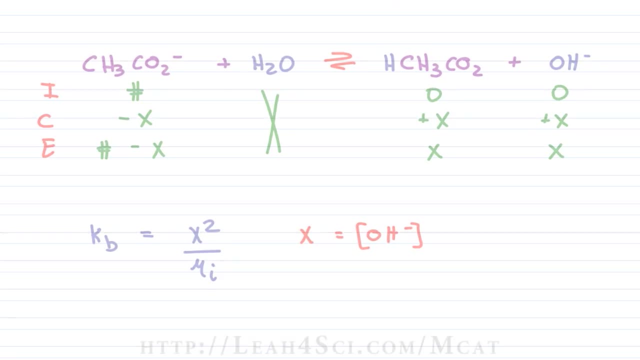 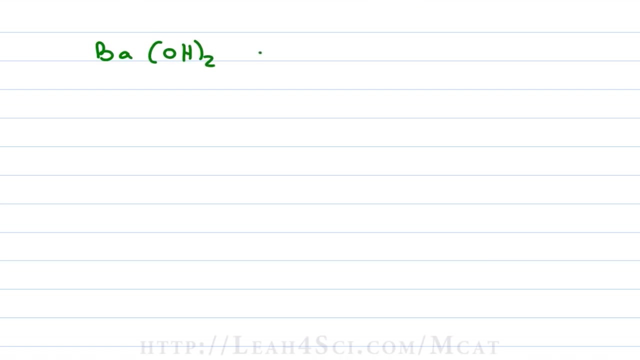 we have a basic solution. We'll get a pOH. we can turn that into a pH, but we have a basic solution. We can save the same thing for strong and weak bases. For example, if I have a strong base like barium hydroxide and I dissolve that in solution, I'll get Ba2+ 2OH- that's how we know. it's a. 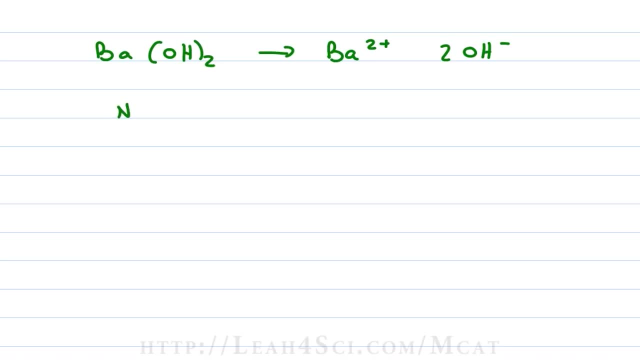 strong base. If I take a weak base like ammonia and react it or dissolve it in water, then I will get at equilibrium NH4 plus as the conjugate acid- OH- as the conjugate base, or ammonia hydroxide if you want to put it together as one molecule. But now the question is: what if I start? 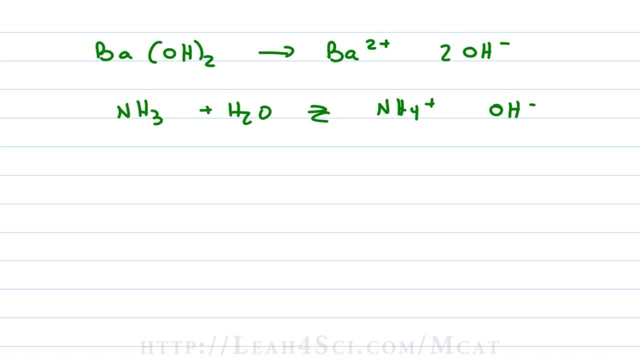 with just the conjugate barium and ammonium and dissolve them in salt version. what happens to the pH? Let's use an anion that we know is not reactive, like nitrate. How do we know nitrate is not reactive If HNO3 is a strong acid and dissociates? to give me H plus and NO3 minus. 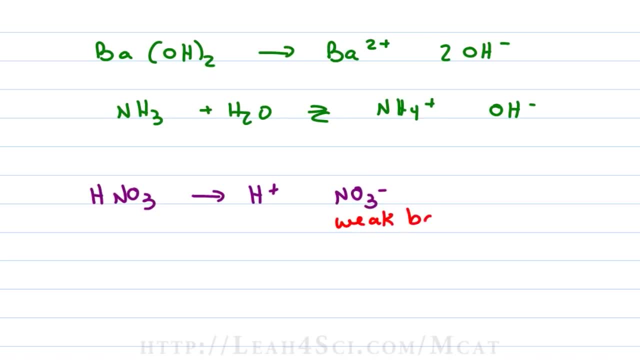 we know that NO3 minus is a very, very weak base because it's the conjugate of a strong acid. So let's see what happens. if we take barium nitrate, BaNO3 2, and dissolve that in solution, We'll get Ba2 plus and 2NO3 minus. both are weak, both are not gonna do anything to the solution. 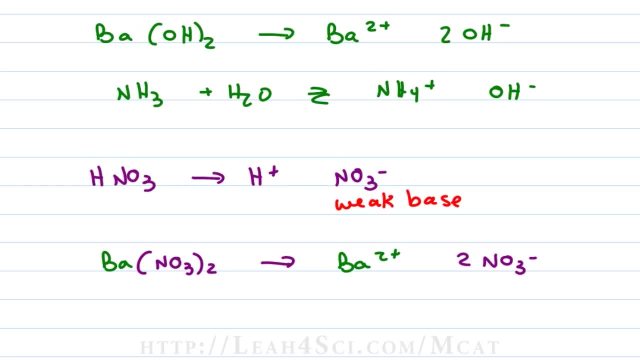 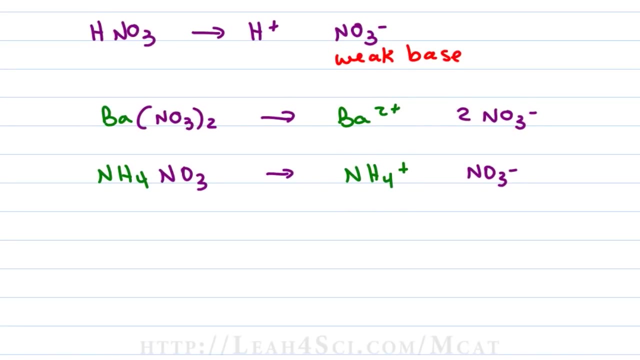 But what happens if I take the conjugate acid of my weak base, ammonium, and dissolve that as ammonium nitrate in solution? Ammonium nitrate will break down to give me ammonium and nitrate. but because ammonium is the conjugate acid of a weak base, it has acidic properties. In fact, ammonium will react. 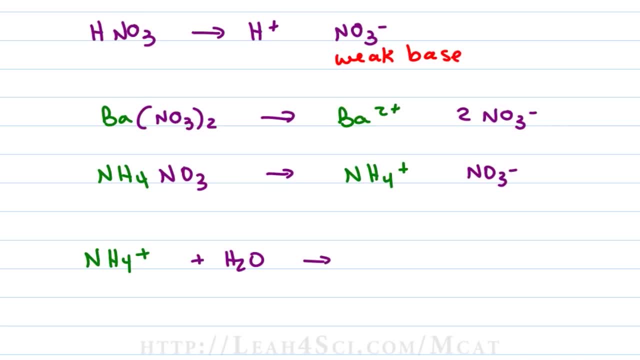 in water, or think of it as reacting with water to give NH3 plus hydronium, which is H3O plus, where the third hydrogen came from ammonium. We have four hydrogen here and two, for a total of six H2O And N2 is N3.. We have to calculate the total levels, so this problem has to be solved. by presenting the lag problem right, Or this vision alone that we had in previous question. here also we can solve the lag problem, and we told you that thels not comes from no OH2.. Here's the problem. you can add this problem a second time so the result wouldn't come true: no OH2,. 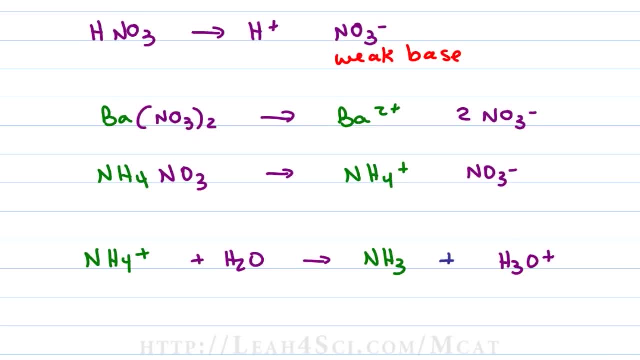 right, but no OH2,. to solve the question último, we can do the follows inconclusive solution which We have: 3 and 3 once again, for a total of 6.. Hydronium is an acidic species. If you take out the water and just write ammonium is breaking up, you'll show it as NH4 plus. 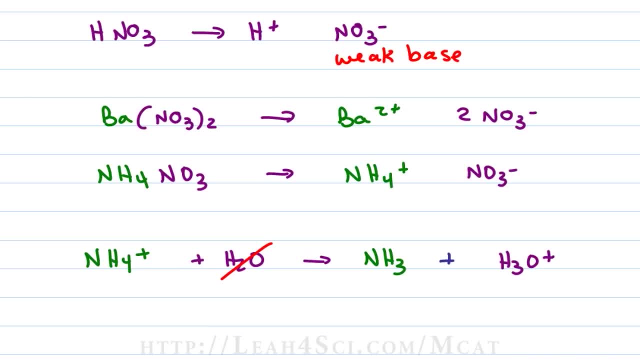 goes to NH3 plus H plus, but H plus and H3O plus are interchangeable. that's why I'm showing it as hydronium, and this is an acidic species, which means you'll have an acidic solution or pH that's less than 7.. 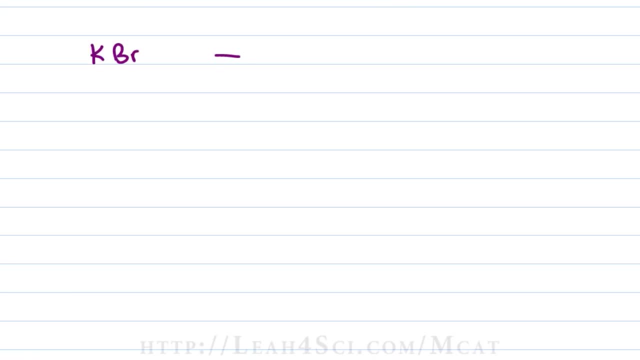 But now what happens? if I give you a salt like KBr? We know that it breaks up to give K plus and Br minus, but is this considered acidic or basic? and how do you know? The key here is to ask yourself: if each ion dissolved and reacted with water, what would 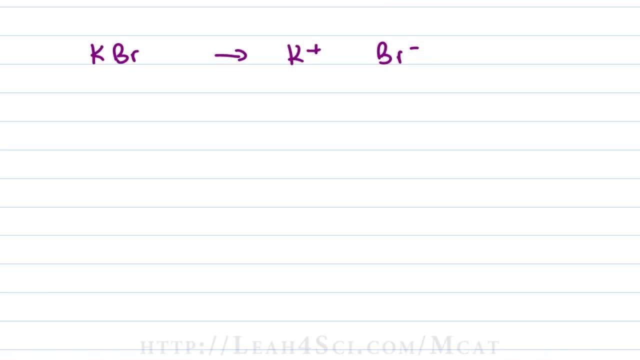 happen and is it strong enough to do that? In the beginning you'll have to go through this mentally and actually work through the reactions, but after a while you'll get pretty confident so that you can simply look at it and understand. If K plus reacted with water, we would get KOH plus H plus. 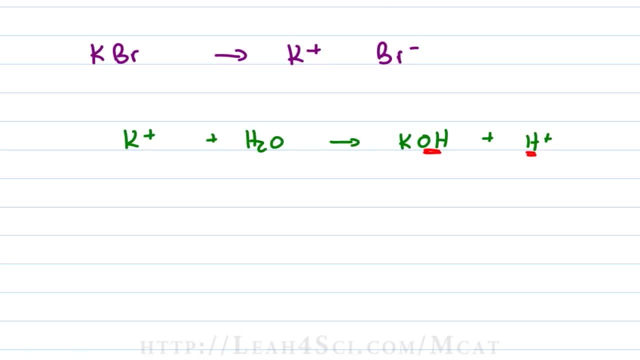 That's because the water broke apart to give me an OH minus and an H plus. The problem is that KOH is a strong base and the reaction will actually favor the reactants, the K plus and H2O, which means that K plus is neutral in solution because it's not strong. 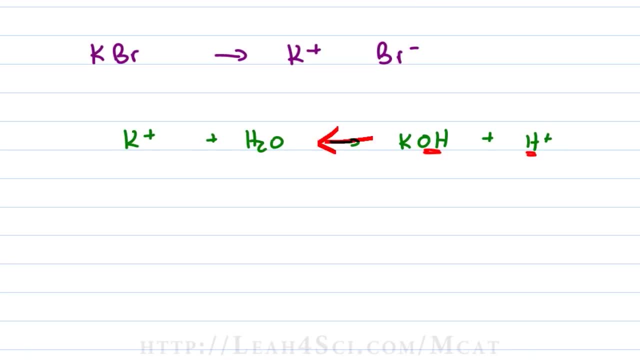 enough to abstract hydroxide from a water molecule. Now let's look at the reaction for Br minus. If we dissolve Br minus in solution, it's negative, so it will grab an H plus, giving me HBr plus OH minus, meaning it would be basic. but once again, HBr is something you should. 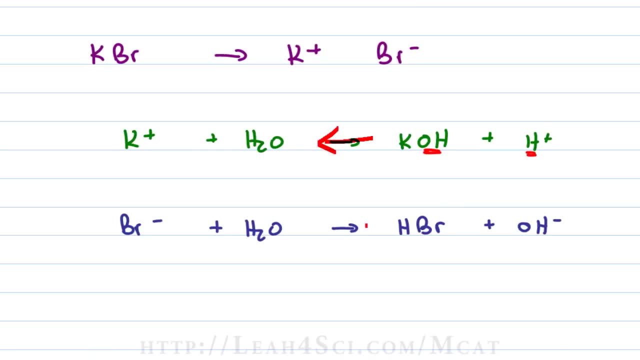 recognize as a strong acid, not something that goes at equilibrium. Once again, we favor the reverse reaction, making Br minus inactive in solution. so if we have a salt that consists of an unreactive cation- Okay, the positive ion, and unreactive anion, the negative ion- then we're going to get a neutral. 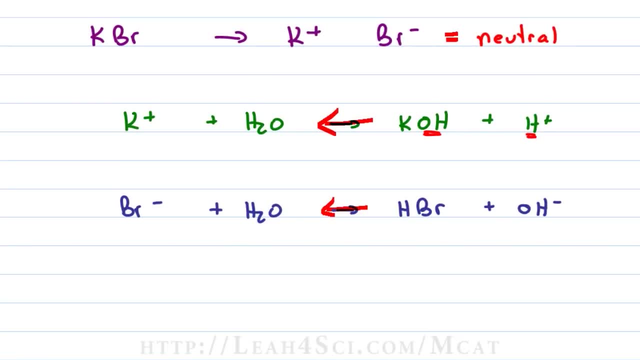 solution because it does not react. So how do you know which ions to look for? Go back to the video on strong acids and strong bases and look at how the ions are set up. Once you understand the acids and bases, just look at their conjugates and recognize that. 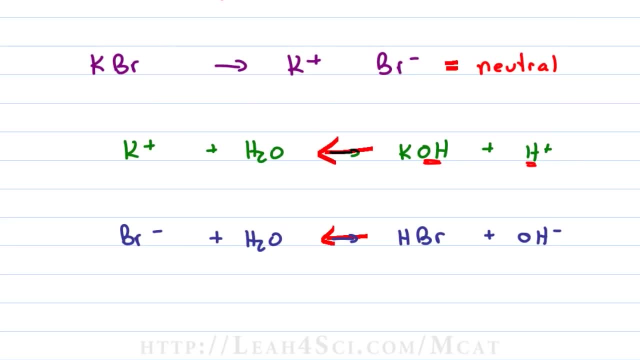 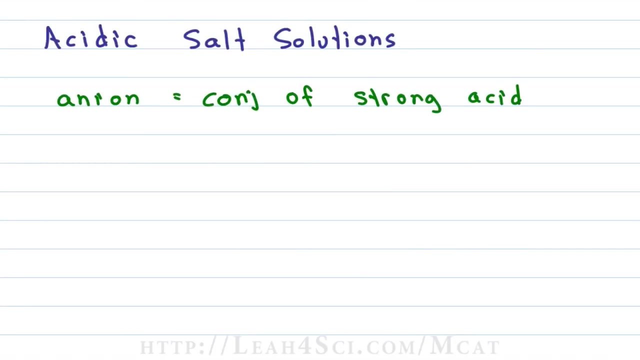 those are not going to be reactive. You can find all the videos, along with the practice quiz and cheat sheet, by visiting my website, leah4scicom. slash mcatacidbase. When the salt in question has an anion that is, the conjugate of a strong acid, it won't. 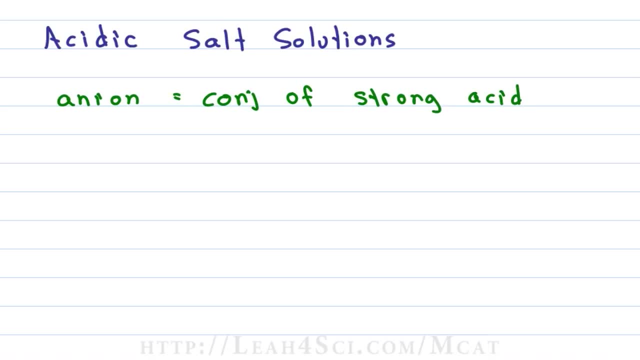 impact the solution because strong acids give weak, unreactive conjugate bases. Those are negative, so they're anions. When the cation is the conjugate of a weak base, we get something positive that is reactive in solution And that will result in an acidic pH. 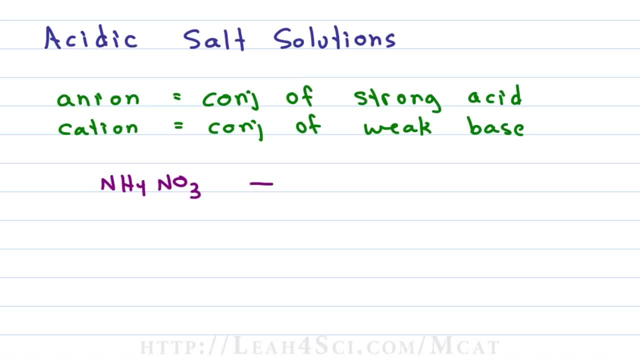 One more time. let's look at the example of ammonium nitrate. Ammonium nitrate breaks up to give NH4 plus and NO3 minus. NO3 minus is the conjugate of nitric acid, which is a strong acid, giving me a weak, unreactive. 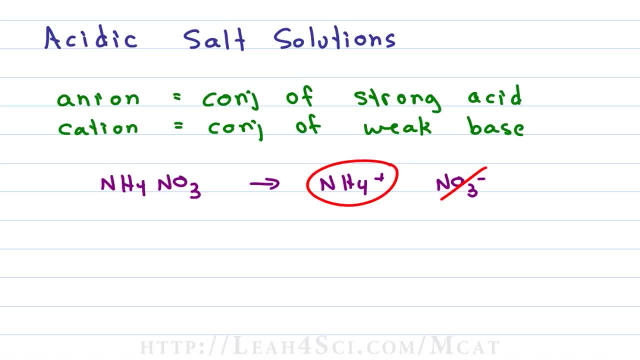 conjugate base, But ammonium is the conjugate acid of ammonia, a weak base, and ammonium will break up further in solution to give me H pluses. Then after ethylene nitric acid or hydronium, making it an acidic salt. 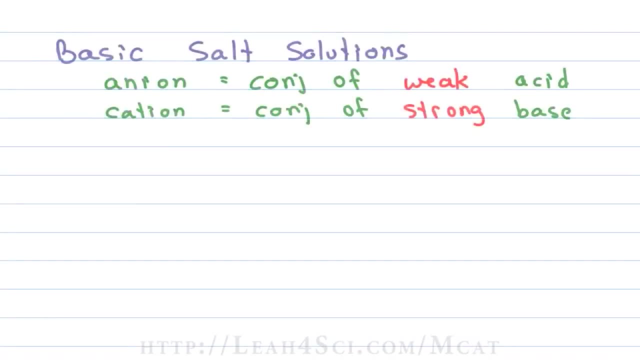 Ammonium nitrate and similar salts are considered acidic salts. Basic solutions are the exact opposite. If the cation in the basic solution is the conjugate of a strong base, that means it's going to give you a weak conjugate acid or a weak positive ion for the cation. 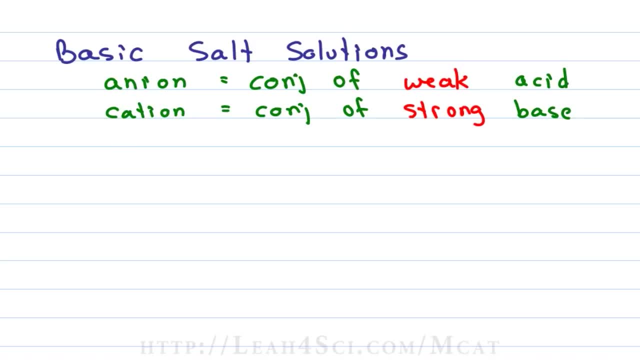 That will not be reactive in solution. And if the anion is the conjugate of a weak acid, that means that these two will not be reactive in solution. If the cation in the basic solution is the conjugate of a strong base, that means it is. 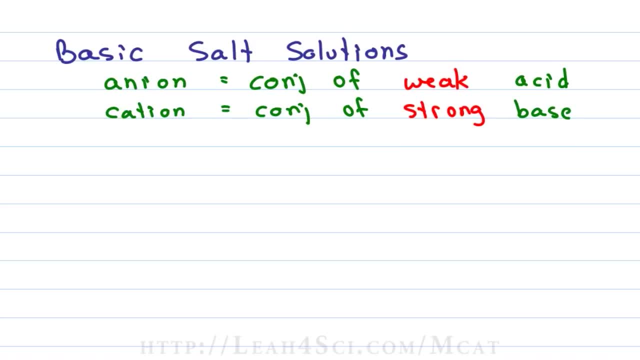 acid. well then, the conjugate of a weak acid is reactive in solution and it will be basic in solution. For example, if we have a salt like KCN, that will break up to give us K plus and CN minus. K plus would react in solution to give KOH, but KOH is too strong. that means K plus is. 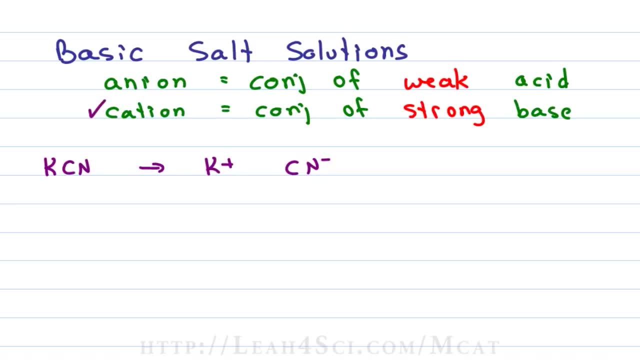 weak, not reactive. that's our cation conjugate of a strong base, but CN minus is the conjugate of a weak acid. HCN will break up in solution and at equilibrium give us H plus and CN minus. Equilibrium tells us it's not strong enough to completely dissociate and instead goes. 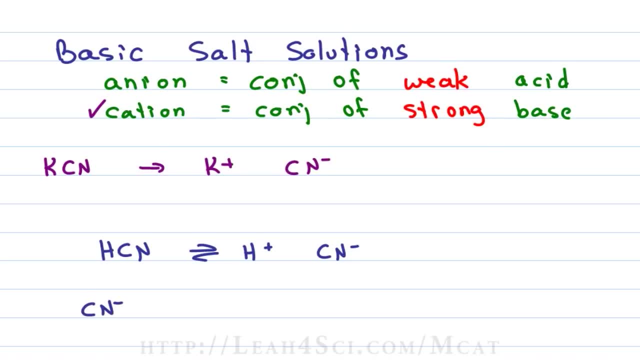 back and forth. So if we take this CN minus in solution, it will react with water and at equilibrium will give us the weak acid HCN plus the left over OH minus hydroxide will give us a POH or simply a pH that is greater than H. 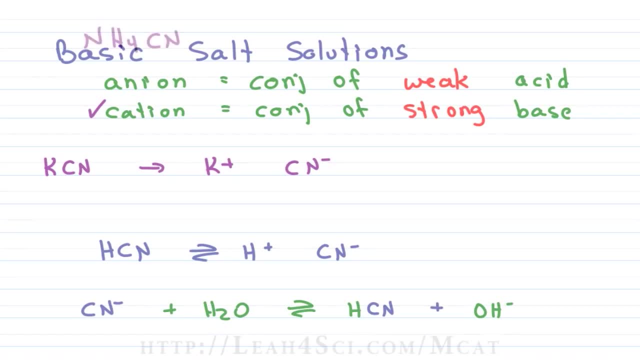 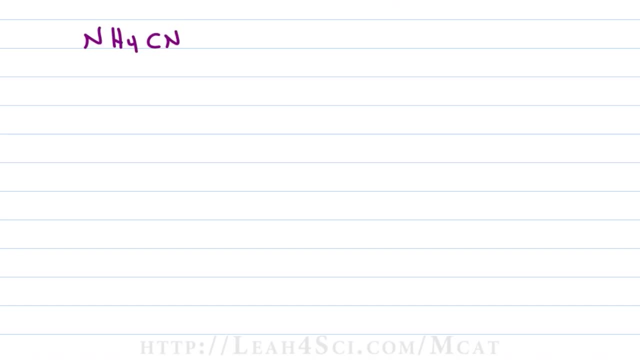 Greater than 7. that is a basic solution. Now what happens when both the cation and anion are the conjugates of weak acids and bases? For example, ammonium cyanide will break up in solution to give NH4 plus and CN minus. 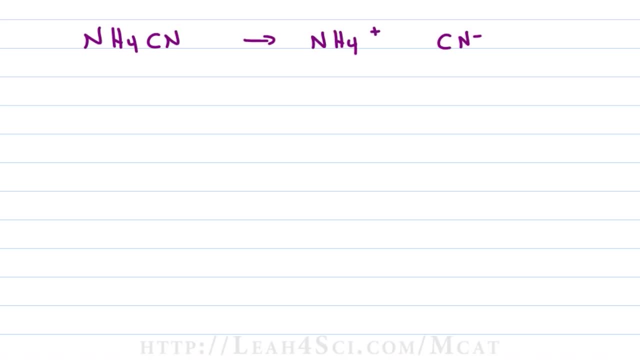 If we look at each one. ammonium is the conjugate of a weak base- ammonia. that would give me an acidic solution, But cyanide is the conjugate of a weak acid, cyanic acid or hydrogen cyanide, which means we would expect to have a basic solution. 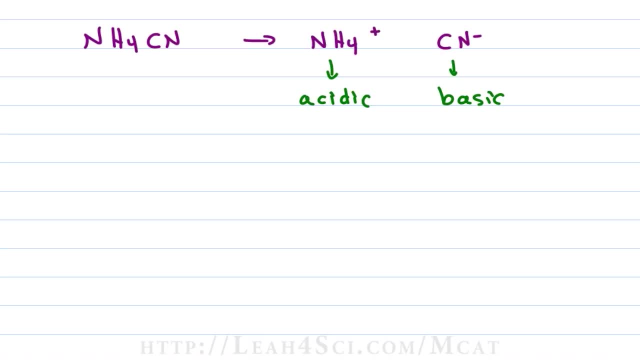 So which one wins? Now, if it comes to math, I don't think this would show up on the MCAT because the calculations would be too involved, but if you're given values of KA and KB, you can compare them to determine which one is going to win, in this case, which one is stronger and therefore 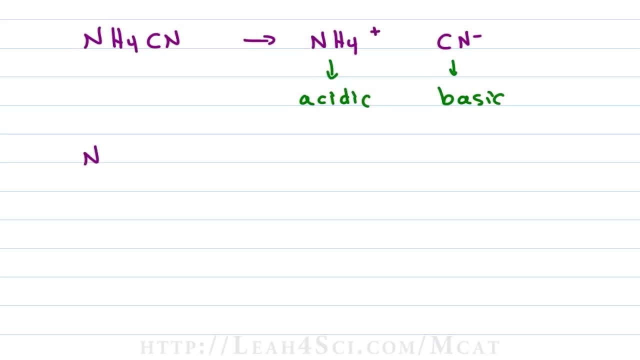 wins the acidity or basicity of solution. Since ammonium is an acid, we would have to look at the KA and remember that KA is proportional to acid strength. The higher the KA, the stronger the acid and therefore, if we have a high KA, we are going. 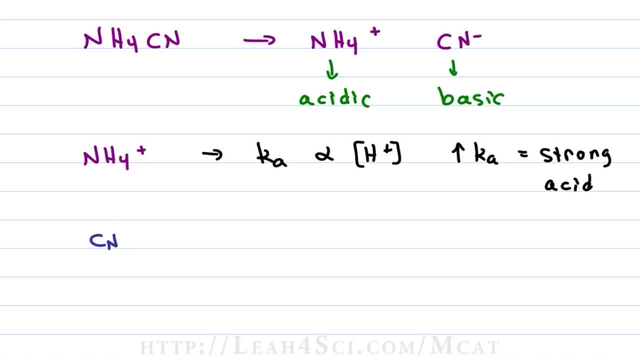 to have a strong acid Cyanide. CN minus is a base. that means we'd have to look at the KB, remembering that KB is proportional to OH minus concentration. So we're going to have a strong acid Cyanide. CN minus is a base. that means we'd have to look at the KB, remembering that KB is. 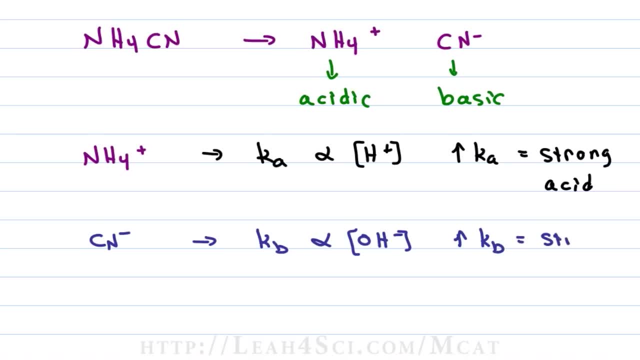 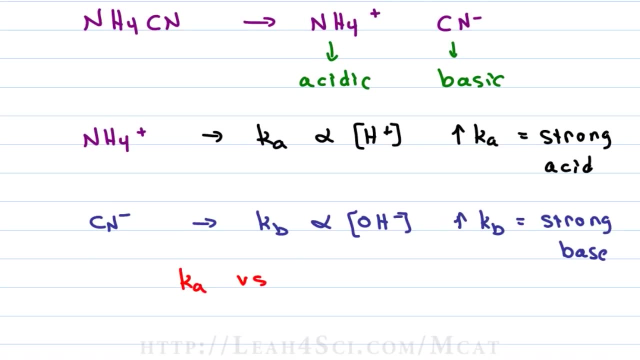 proportional to OH minus concentration, Telling me that the higher the KB, the stronger the base. If you're given these two values, simply compare KA to KB. If the KA is greater than the KB, it tells you that the KA is more powerful at directing. 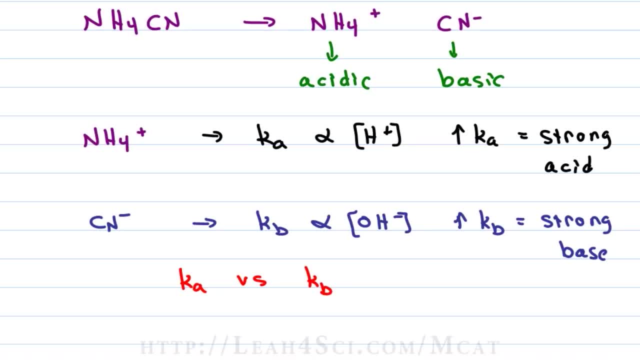 this solution and therefore it's going to be acidic. But if the KB is greater than the KA, that means the base is stronger. the base wins out and it'll be a basic solution. How to calculate the actual pH or pOH requires too much math and I doubt it will show up. 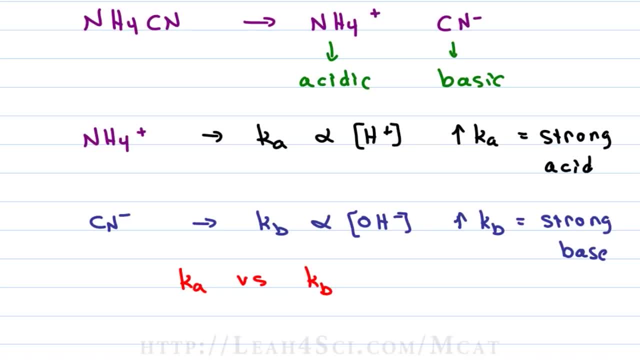 on the MCAT, but you should understand the concept in case you're asked to analyze a question without numbers, but simply ask for concept. This concludes the MCAT acid base series. Remember you can catch the entire series, along with the practice quiz and cheat sheet, by